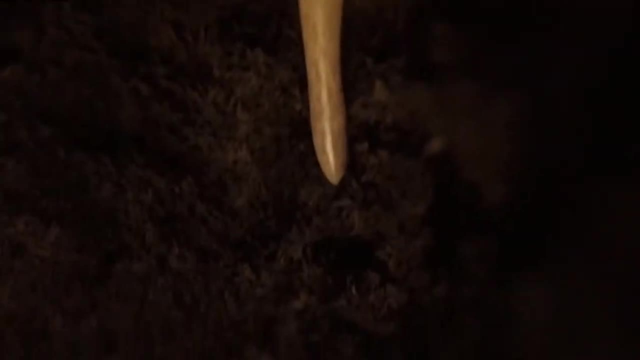 They don't live long, only 1-3 weeks, As you can see, they don't live long, only 1-3 weeks. As you can see, they don't live long, only 1-3 weeks. As you can see, plants need external help. 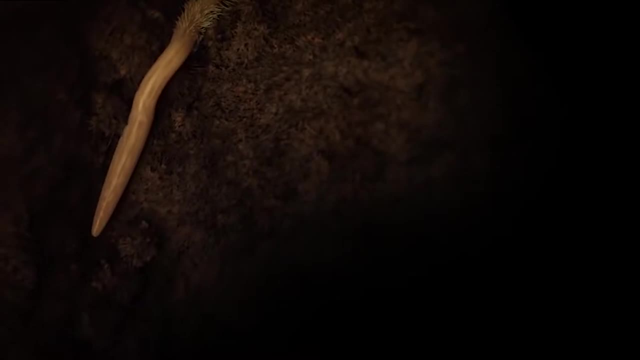 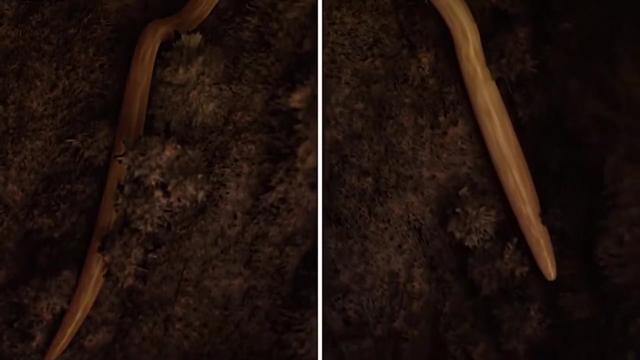 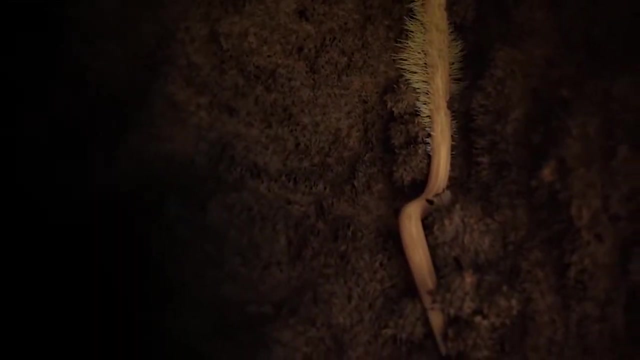 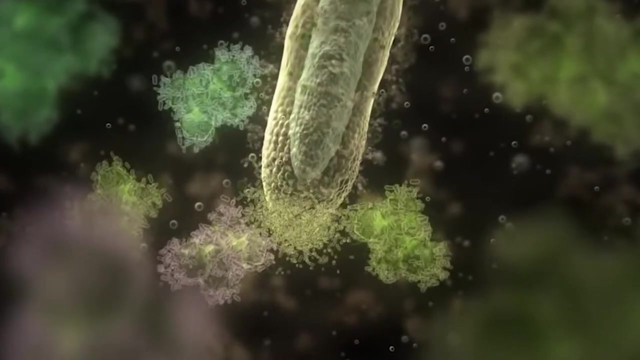 Plants use their absorption roots to forge a partnership. If they can't find partners, they'll die. If they succeed, it's the start of a beautiful relationship. From now on, a symbiosis can be created. Minerals are hard to mine from the soil, but rhizobacteria are specialised in this process. 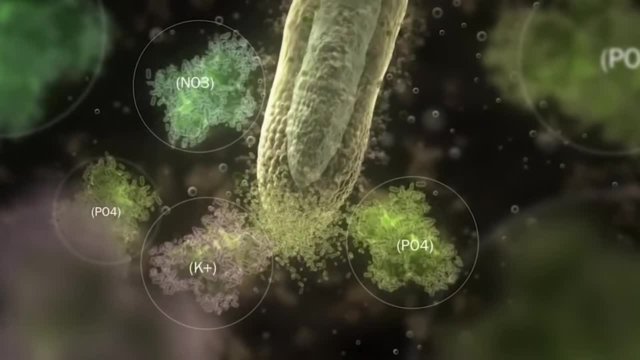 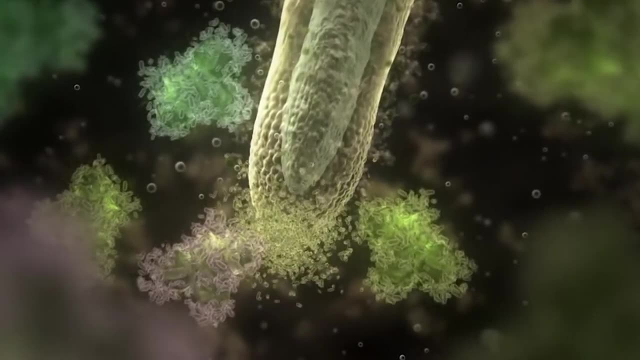 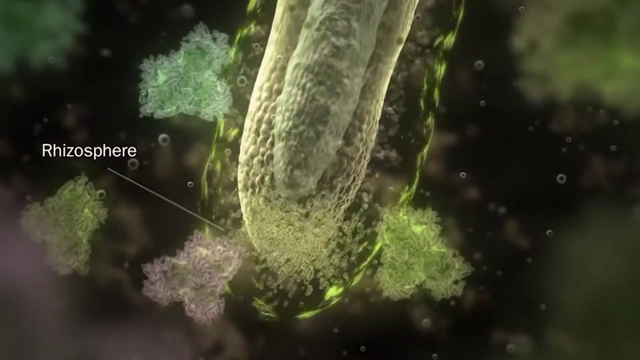 particularly when it comes to the soil, When it comes to releasing phosphate, which is very important for the plant. these bacteria also carry out countless other important tasks, including one which is very special: Rhizobacteria form a sort of natural defence system around the roots. 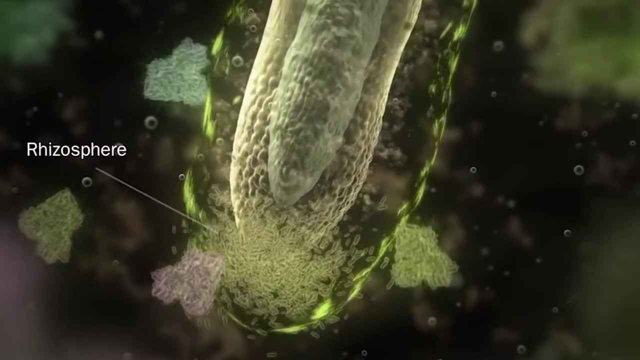 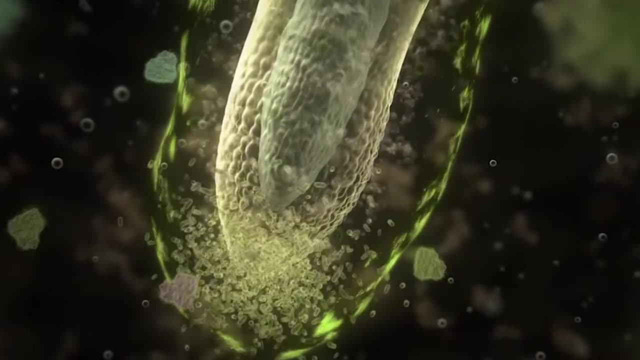 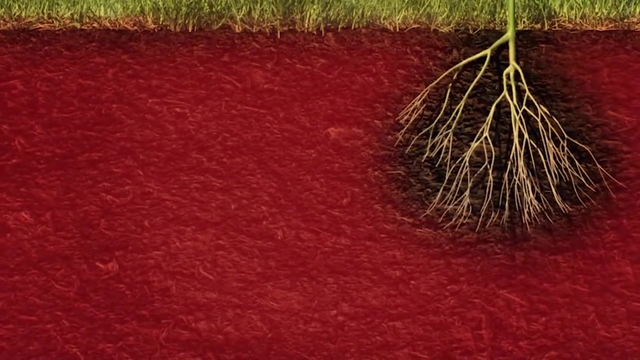 Anything attacking the plant is kept outside by the physical presence of these rhizobacteria. They ensure that there is no room for disease-causing bacteria. They have their own interest in this because the plant provides them with food. However, the bacteria also need help. 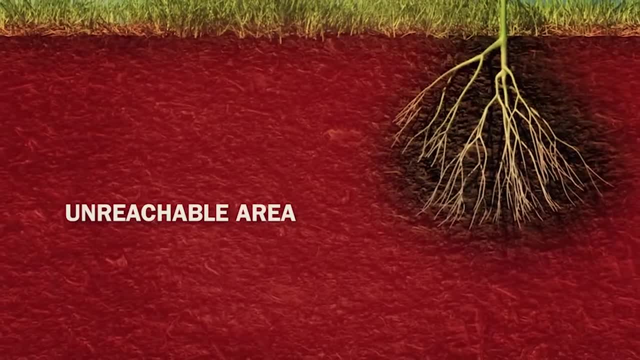 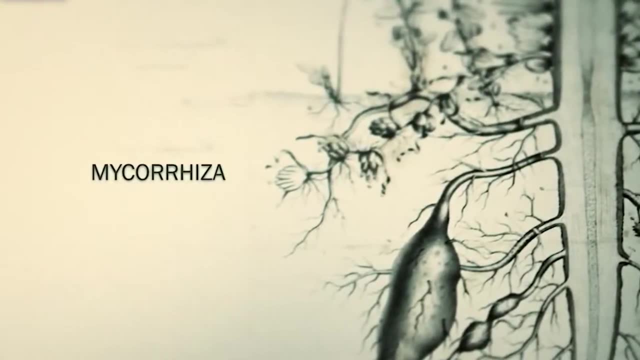 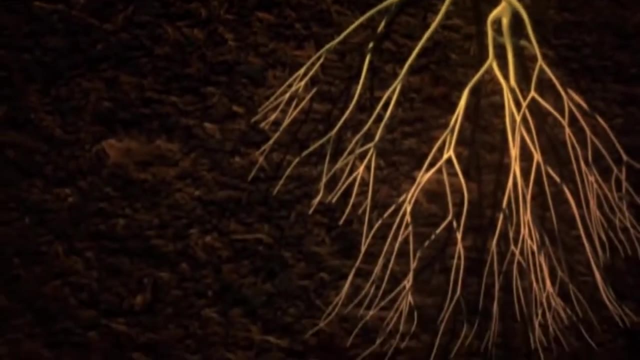 They are not travellers. The bacterial colonies do not move back and forth from minerals to the roots. Most minerals found in soil are located outside the reach of the roots and therefore also out of the reach of rhizobacteria. These can only live near the roots. 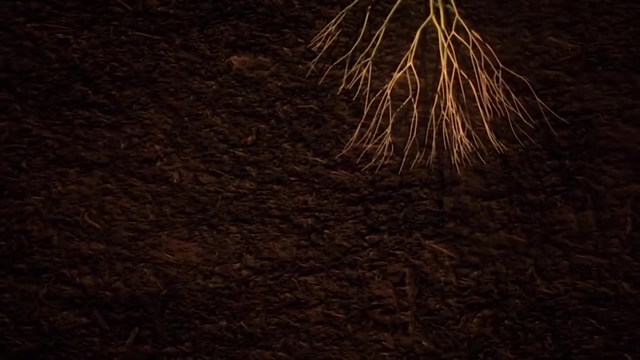 As we have seen before, the zone of absorption is therefore very important. As we have seen before, the zone of absorption is therefore very important. As we have seen before, the zone of absorption is therefore very important. Mycorrhizal fungi are able to drastically increase this absorption capacity. It may sound like a modern development, but it's not. The fungus has always existed, but due to modernisation, its role has been neglected. Due to many years of using synthetic fertilisers, mycorrhiza is only very sporadically found in agricultural soils. 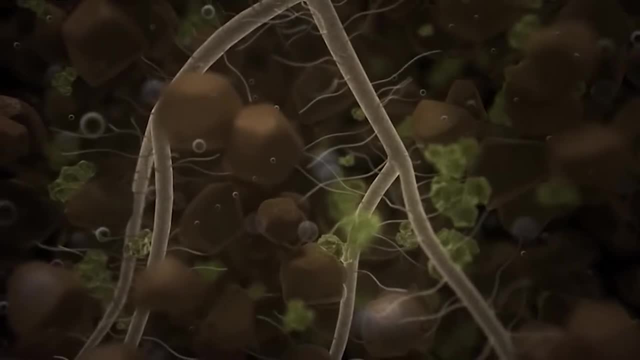 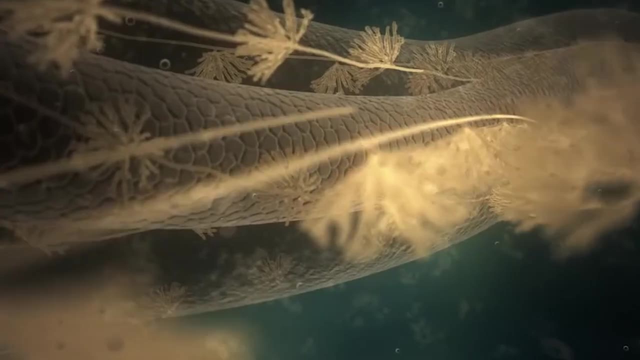 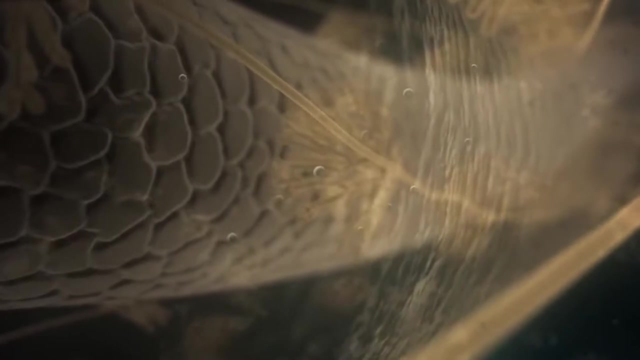 Mycorrhizal fungi have always lived in simple, in symbiotic relation with the plant roots. Mycorrhizal fungus forms a living connection within the roots and creates an absorption and transport system. This is essential for healthy plant growth. Mycorrhiza in the roots is just as normal as chlorophyll in the leaves. 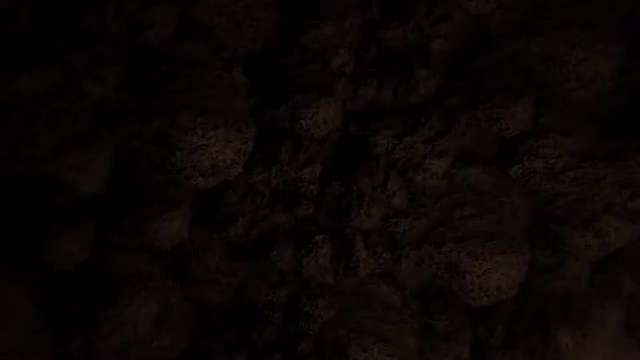 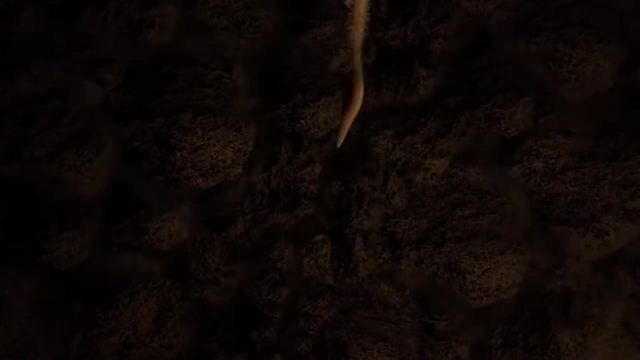 This is beyond doubt. As stated before, the absorption roots of plants are 0.2 mm thick. This means that they can only grow in macropores, as shown here. Now we zoom in to see what happens when the plant gets help from the mycorrhizal fungus.